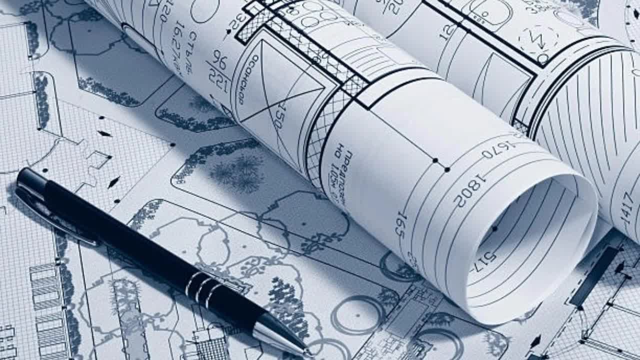 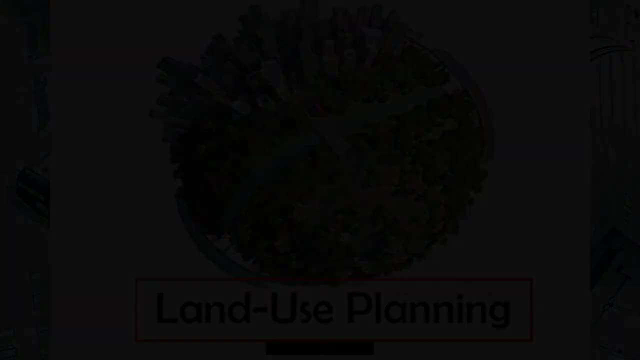 Assalam-o-Alaikum, beautiful people, Welcome back to e-sabak. Myself, Rehan, and today we are here with a new tutorial. In this tutorial we will discuss land use planning. In this module, the learning objectives are central: idea of land use planning, need for land use. 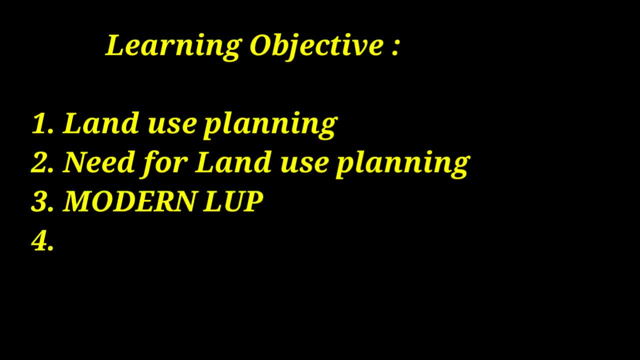 planning, modern land use planning, importance of land use planning, objectives of land use planning. and then, finally, we will discuss principle of land use planning. Guys aajki iss video mein hum, mostly cover karenge tiin cheeze. definition of land use planning ki. 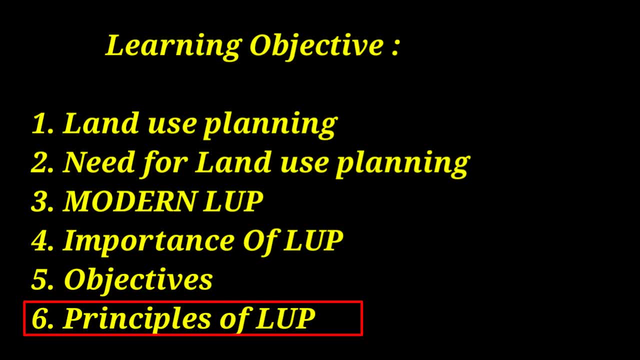 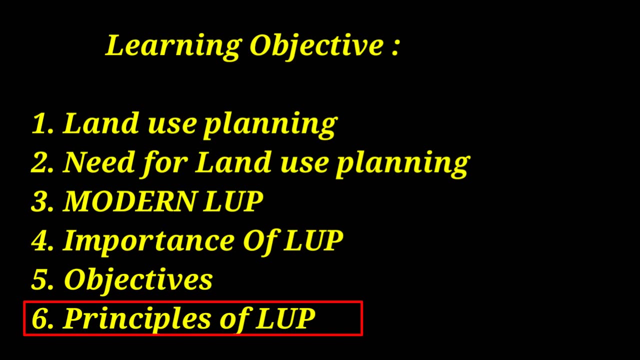 ye land use planning hoti kiya hai aur hum kyon karte hain land use planning, Then hum study karenge objectives of land use planning And then, finally, we will discuss principle of land use planning and in our next session we will study methods and techniques for land. 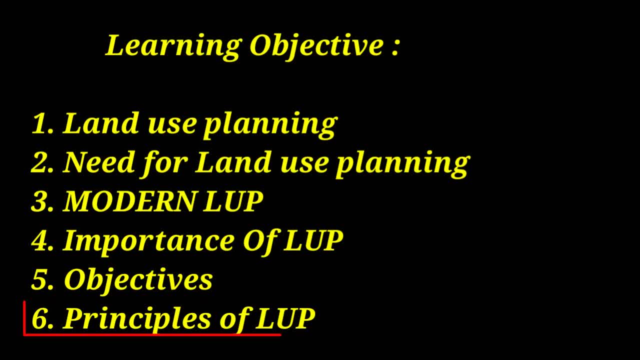 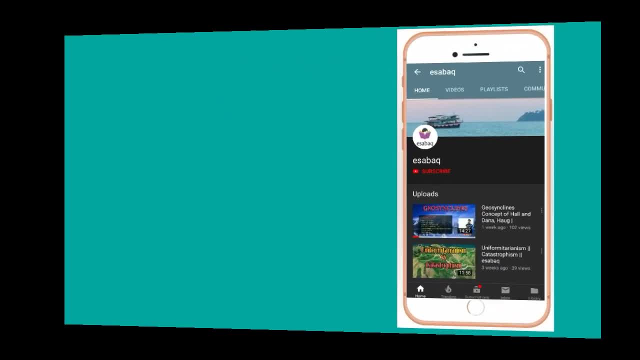 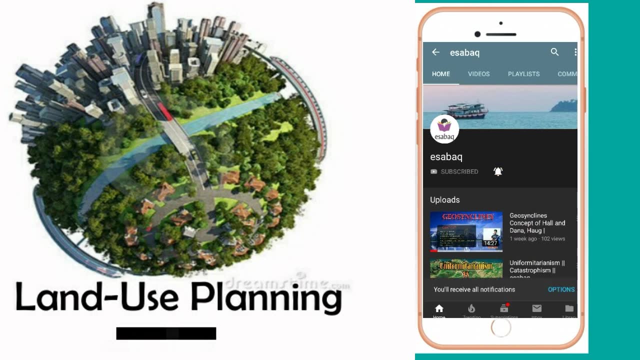 use planning and land use planning in India. So, guys, to understand this concept, to clear this concept, watch our videos till the end And, friends, subscribe to our channel and turn on the notification bell so that in the future, we will keep you updated on the latest videos. 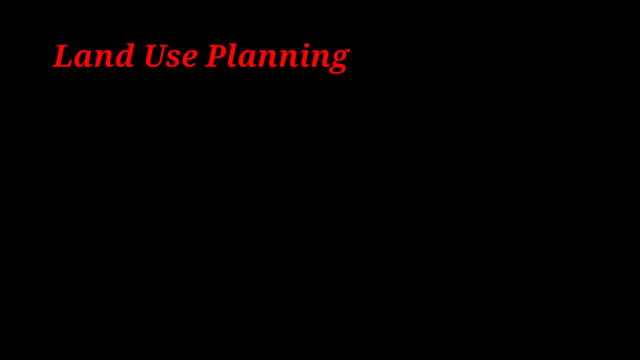 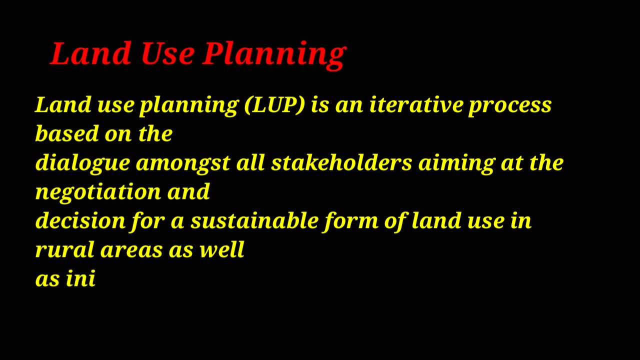 Alright, guys. first let's see the definition of land use planning. Land use planning is an iterative process based on dialogue among stakeholders, aiming at the negotiation and decision for a sustainable form of land use in rural areas, as well as initiating and monitoring its implementation. 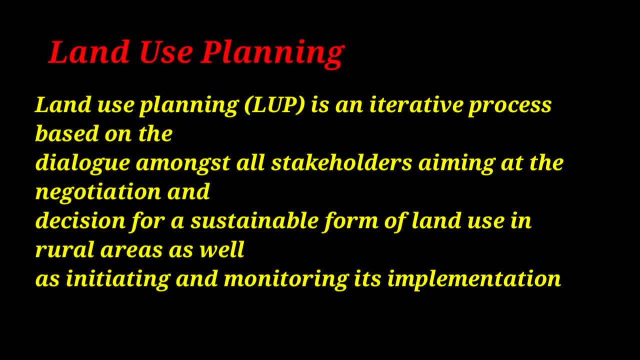 So land use planning is a process of planning and implementation. So land use planning is a process of planning and implementation. So land use planning is a process of planning and implementation. A land use planning is an iterative process that keeps repeating. quickly. A plan can give you a minimum of 5 to 20 years. 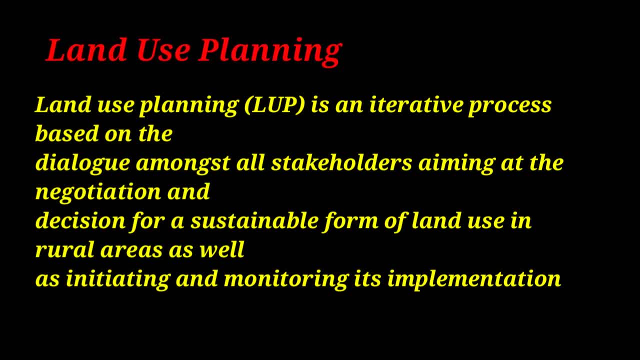 A. land use planning is a process. that is re Musicalание, That is repusle to the dialogue. That is a cocky process here select a and then they have a dialogue that becomes a plan. that then again to the plan, that is aim presentation, and then they 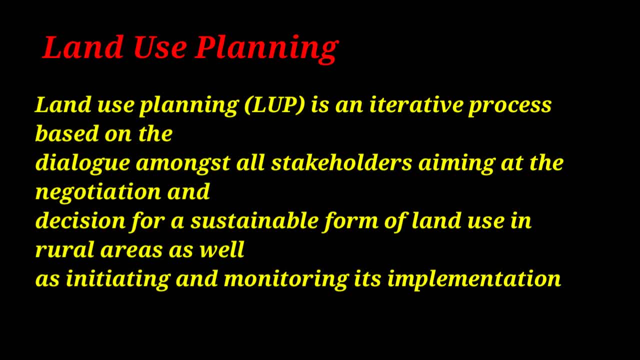 come upon the different stakeholders as a directement nickel. We will make a plan by which we will use our land in a sustainable way so that we can also take advantage of it, and our future generation should not have any effect on its resources. they should also take full advantage of it. 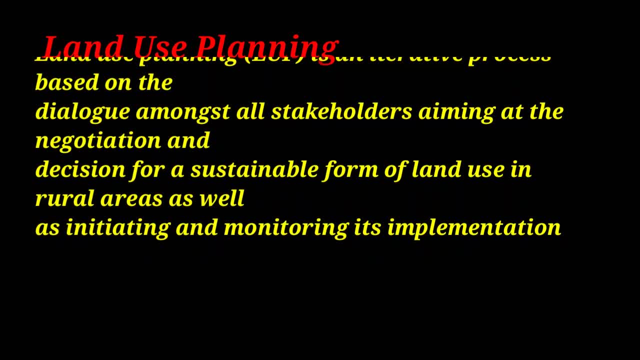 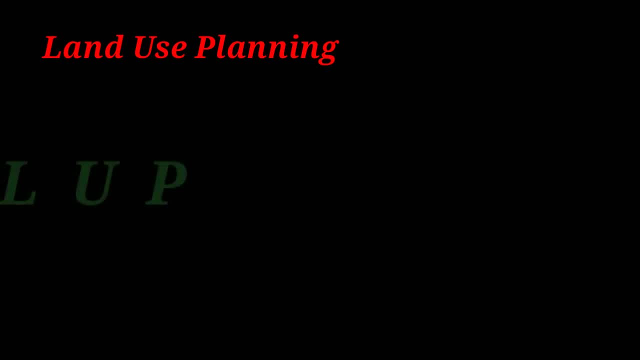 And then when they make a plan, the government is responsible for it to act on it and implement it. Land use planning is denoted by LUP in abbreviated form: L stands for land, U stands for use and P stands for planning. 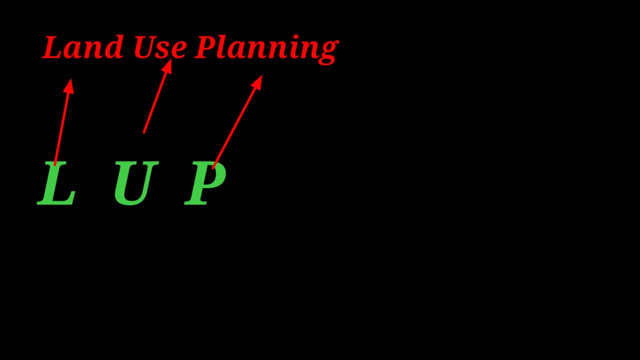 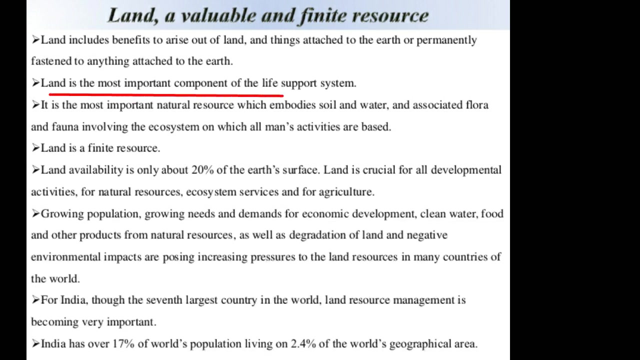 So the combination of LUP includes land, land use and organizational space. in future, Let's define land first. Land is the most important component of life support system, And what do we know about it? Land is a natural resource and it is gifted from Allah. 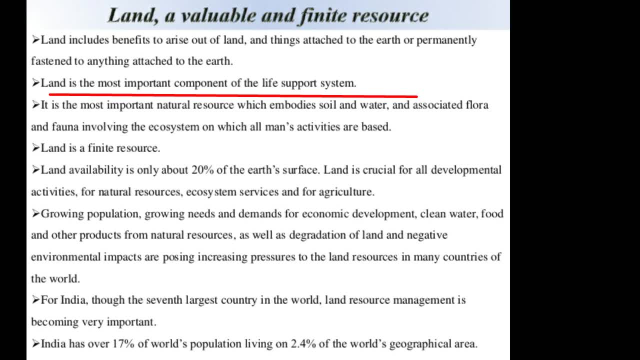 So land is the name that God has given us, and land is the basis of our living. It provides food, shelter, filters, stores water and supply space for urban and industrial development. If we look at any urban or industrial development there, the land will provide the space to us. 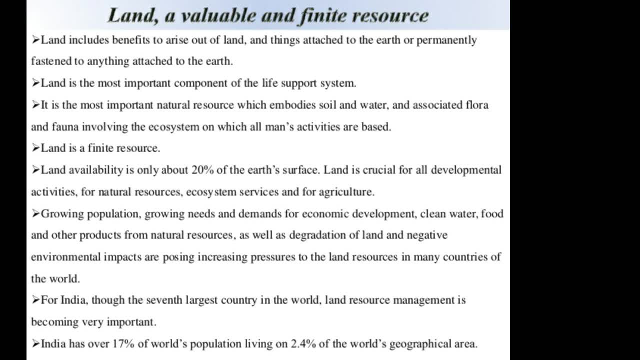 How do we define land? It is the land that is the symbol of life and we like it. the dry part of the earth. Land is a vital resource and an expression of power and wealth. If we look at the rural area, then the land there is an expression of power and 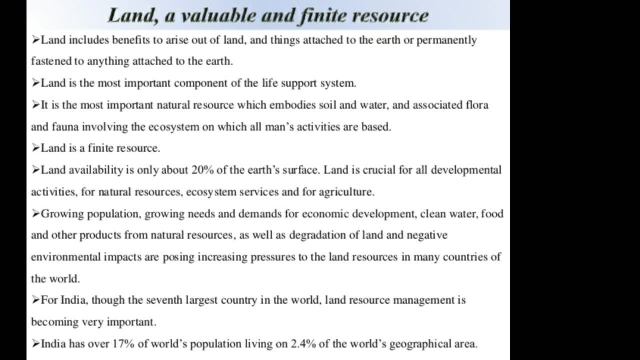 wealth. The farmer who has as much land as he has, he will have as much land and he will be rich there. If we talk about the urban area, then the land is not that much available here. People do not have their own land for production, for cultivation or for agriculture. But if we talk about rural areas, 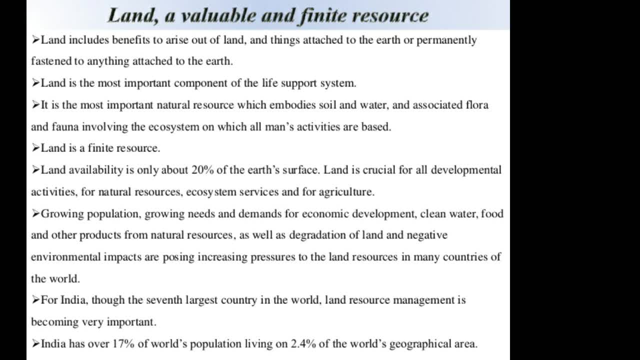 then people there have their own land and do the expression that whatever land they have, he is the king of that place and he enjoys life. so much. Now the important point is that land is finite in extent. Now land is not infinite as much we use. 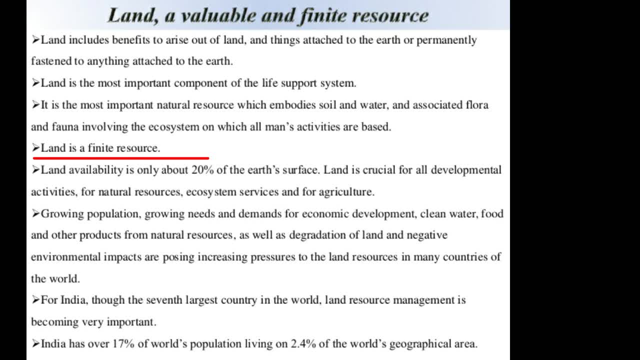 how much we use it illegally, how much we use it in orderly? we will not use it. But the land is finite, it is limited. If you use it correctly, then the land is finite. But the land is finite, it is limited If you use it correctly. 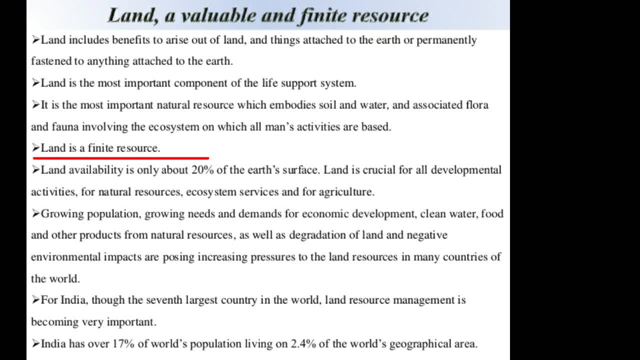 you will be in benefit, and if you use it wrongly, then it will have an adverse effect. as i said, that land is limited in extent, whereas more and more people compete for land. in order to avoid that this competition turn into conflict, firm agreement must be made on how and by 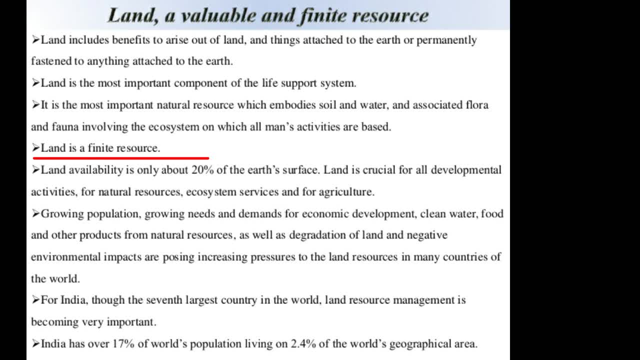 whom the available space will be used. land use planning is a tool to support the orderly occupation and use land and to avoid the adverse development up land was planning how land is put into use by man. for india, though seventh largest country in the world, land resource management is become. 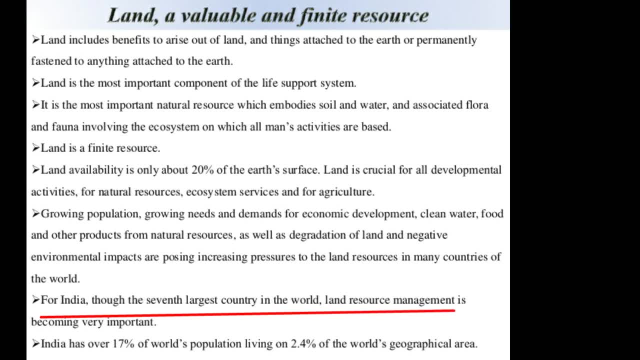 very important and india has over 17 percent of the world population living on 2.4 percent of the world geographical area. india is the second largest uh most popular. we can say that india is the second most populous countries in the world after china. it shares. 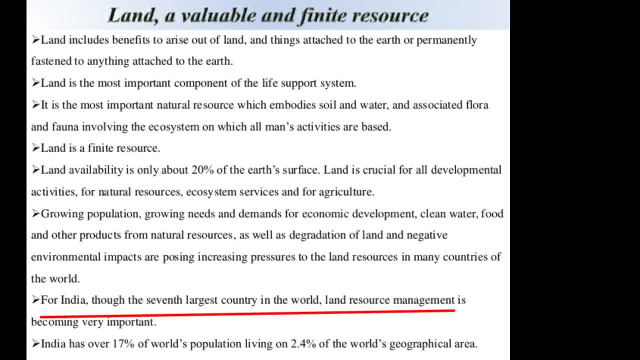 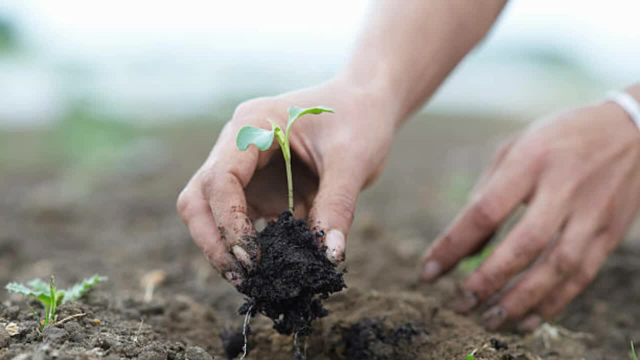 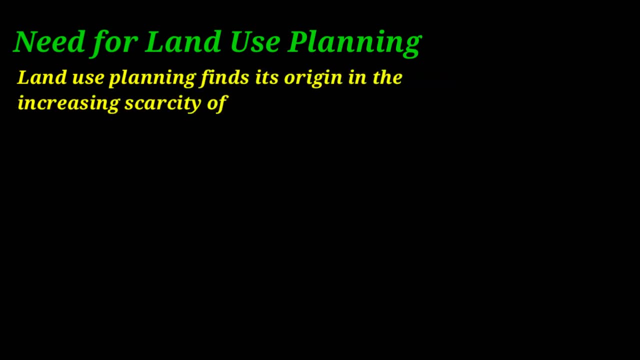 two 2.4% geographical area to the world, and here the management of land use planning has become important. now, coming to the next point, which is need for land use planning. actually, land use planning finds its root in the increasing security of land, the competition for land by growing number of 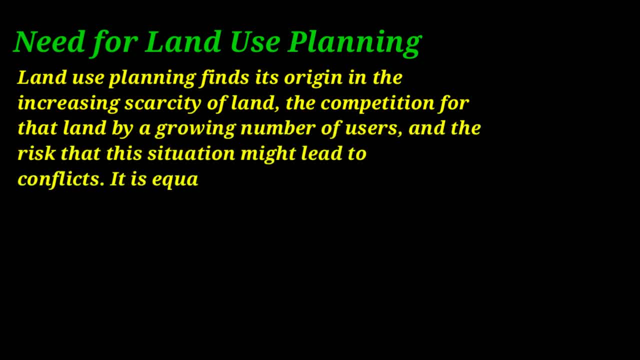 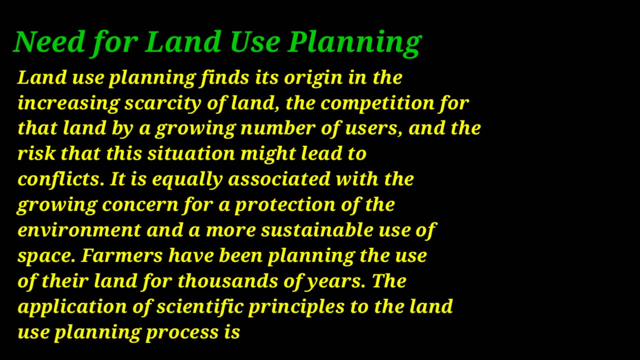 users- we can say that number of population and the risk that this situation might lead to conflict. it equally associated with the growing concern for the protection of the environment and a most sustainable, suitable use of space. we can say that farmer have been planning the use of their land for thousands of years. 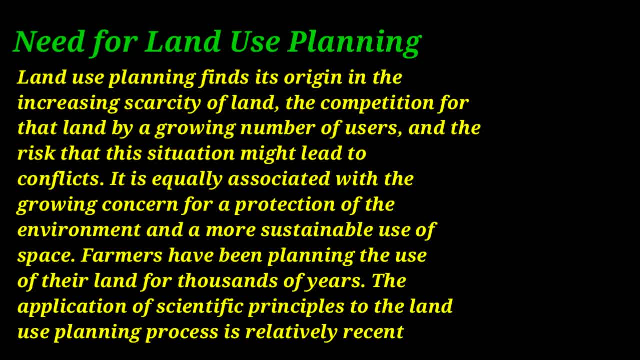 now the farmers are using it for thousands of years. they are planning how to use it, where to do what, where to do horticulture, where to do apiculture. so they are doing it for thousands of years, but the scientific concept and the scientific thinking is recent. 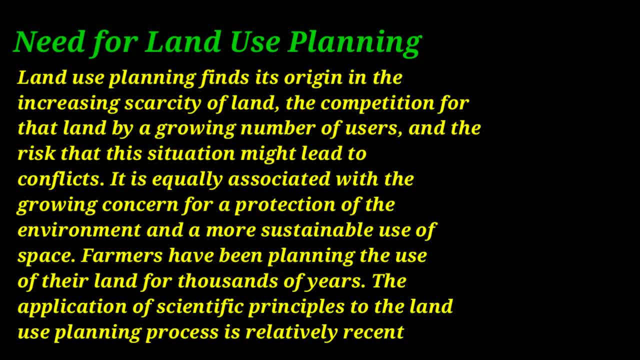 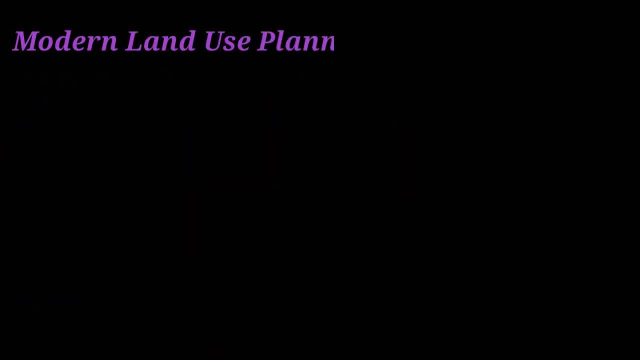 the application of the scientific principle to land use planning process is relatively recent. now coming to the next point, which is modern land use planning. before this we have read that the farmers in India or any other country, they were planning the use of land, but it was not a scientific way. 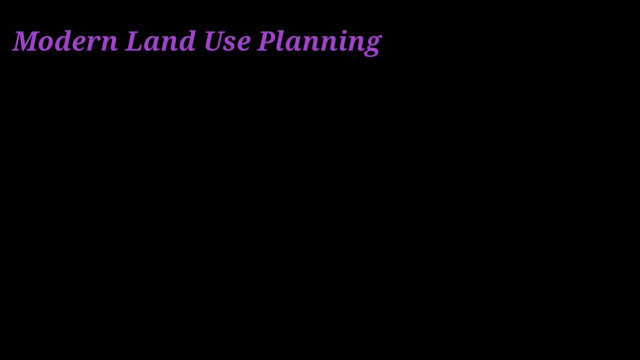 means they were not doing it scientifically, but they were doing it like this. but modern land use planning is always focused on one or more scientific objectives and is closely linked to the land use planning process and is closely linked to the concepts of efficiency, equity and sustainability. 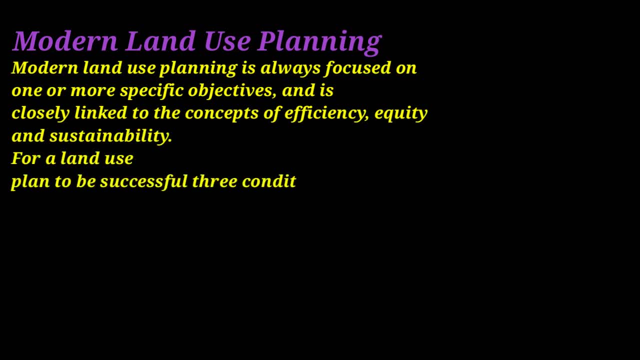 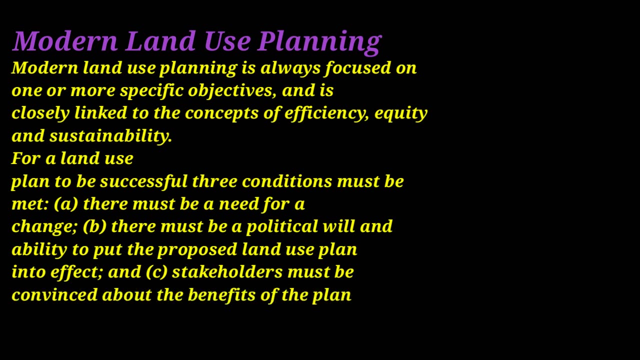 modern concept is the concept of sustainable development. what is in this concept? to meet the need of present generation without compromising the ability of future generation to meet their own needs and demands. for a land use plan to be successful, three conditions must be met now if we make any land use plan. 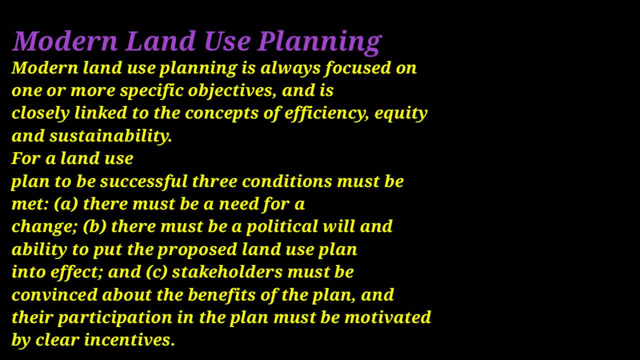 for that it is very important to have three conditions. after that the plan will be successful. the first condition is: there must be a need for change. so the first condition to be satisfied is to change the existing plastic plan. There must be a need for change in the existing plan. 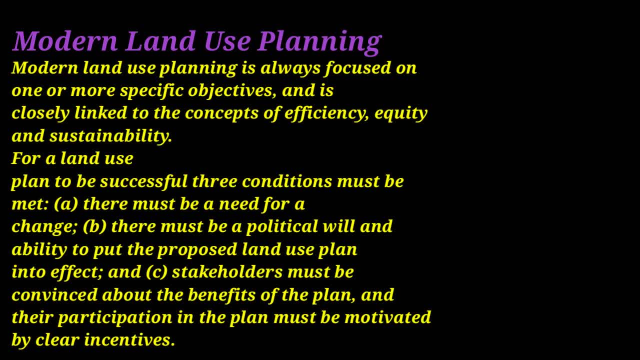 The first condition is that there should be a political will. if we are making a plan, which should be a political will and must be applied to it, And their participants in the plan must be motivated by clear initiatives. And now we will see the elements. Land use planning is based on three elements. 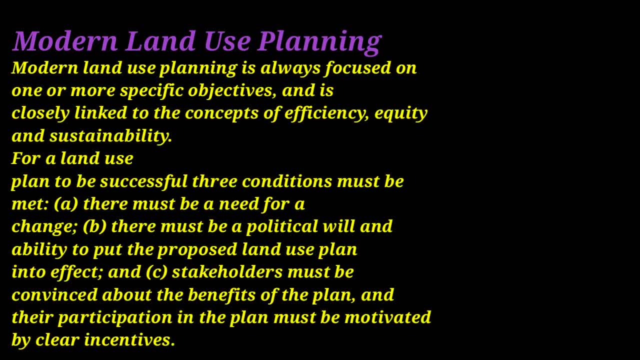 If we see any land use plan, then its elements are mostly three. The first element is long term objective, which sets the overall target of the plan. The second one is strategies for achieving these objectives And the third one is project for implementation, the chosen strategies. 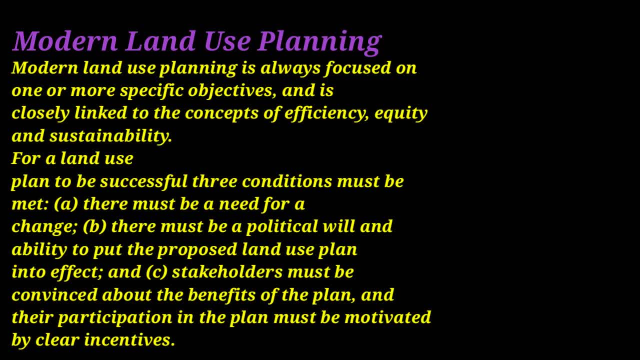 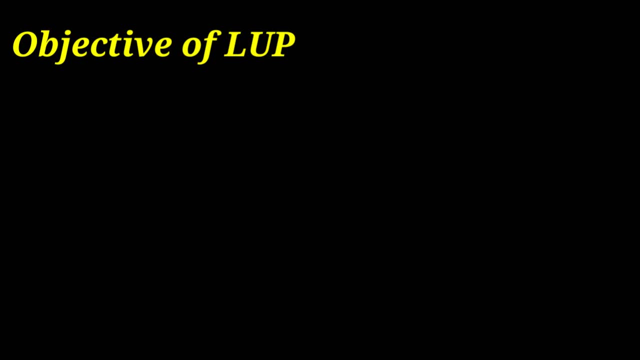 So we have seen that there are some objectives which we have to set and implement. These are the elements. Now we will see what are the objectives in the land use planning. Mostly, if we study, then the highlighted objectives are sustainable development. Our mission is first sustainable development. 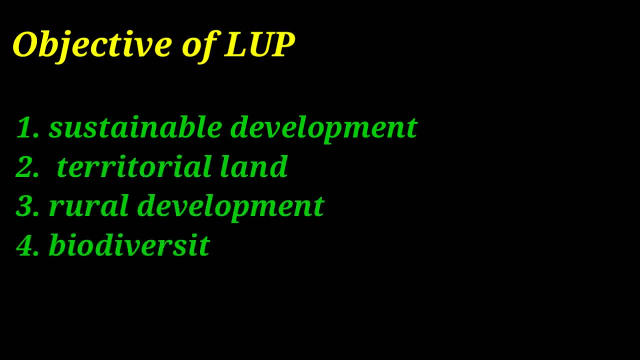 Second is territorial land, Third one is rural development, And the fourth one is land use planning. Fourth one is conservation- biodiversity conservation, And the fifth one is resource conservation and policy. Now to sum up, some of the objectives of land use planning are defined as: 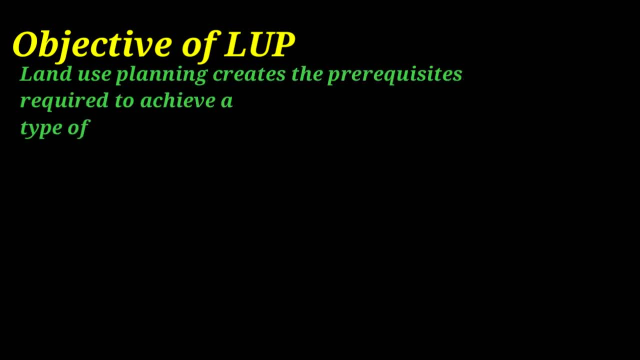 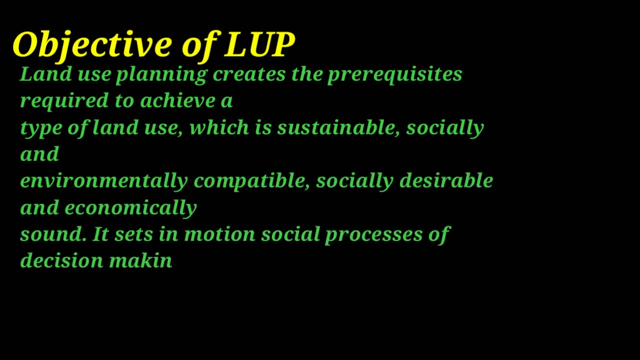 Land use planning creates the preconditions required to achieve a type of land use which is sustainable socially and economically, or we can say environmentally capable, socially desirable and economically sound. It sets in motion social process of decision making and census building concerning the use and protection of private, commercial and public areas. 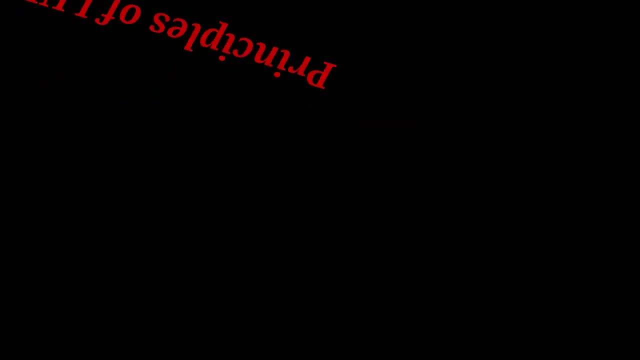 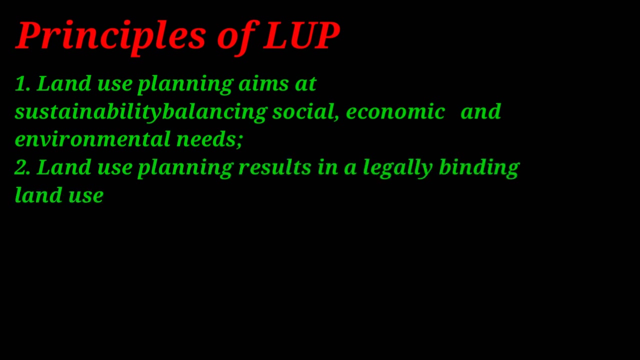 Now coming to the principle of land use planning. The first one principle is: land use planning aims at sustainability, balancing social, economic and environmental needs. Its result in a largely bending land use rules. It is a dialogue. It is based on stakeholder differentiation and gender sensitivity. 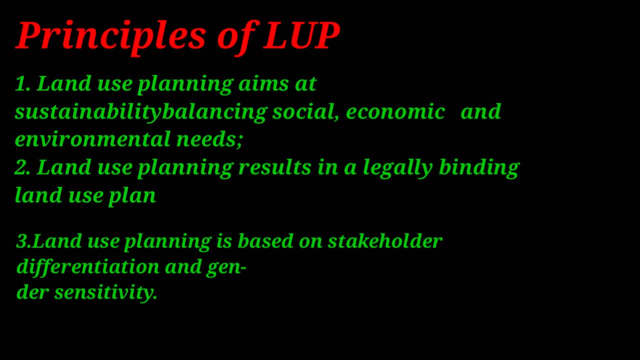 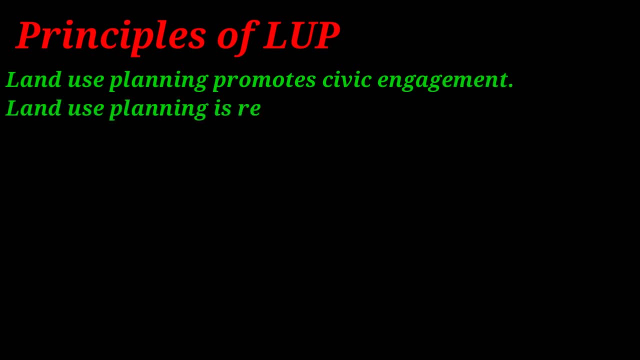 It is based on interdisciplinary cooperation. Land use planning promotes civic engagement. Land use planning is realistic and oriented to local condition. It is based on light methodologies. LUP, in terms of methodologies and content, differs. Land use planning considered and valorizes local knowledge. 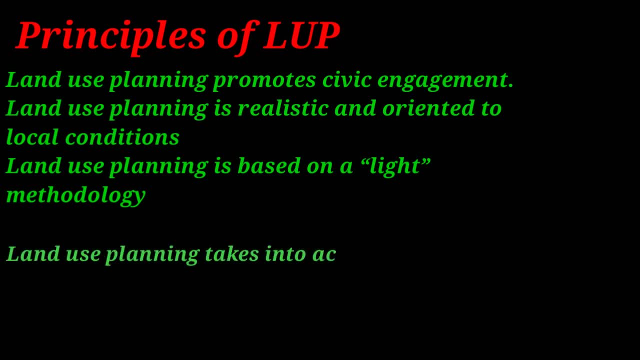 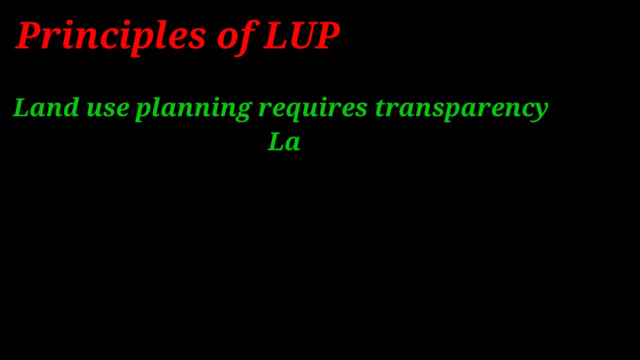 Land use planning takes into account traditional strategies for solving problems and conflicts. Land use planning follows the idea of subsidiarity. It requires transparency. of course. Land use planning is an iterative process. It is a type of plan which is repeated after some time. 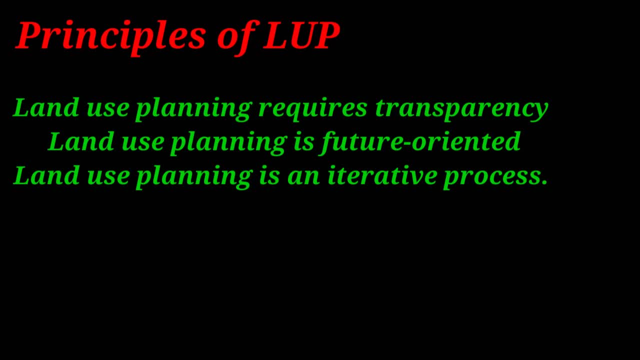 The repetition time might be 5 up to 20 years and the plan will not last up to a century or a decade. Land use planning is implementation oriented. LUP is linked to financial planning, LUP related to spaces and places. So, guys, I hope that you have liked this video. 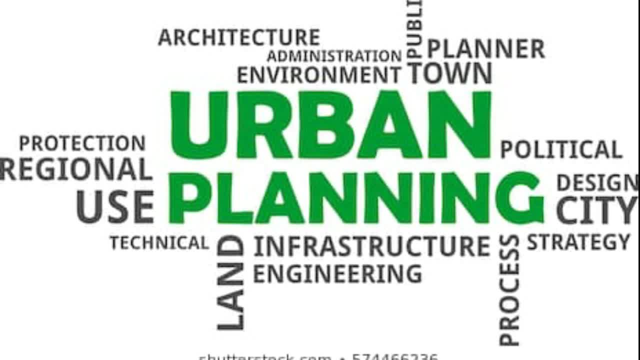 If you have liked this video, then please like it, share it and subscribe to our channel.